that I need that temperature change in order to get heat from that. I don't have enough room to do that right. So Celsius is so important. The simple answer is that refrigerant will get Осmos in those temperatures. I'll get that again. that will make particle loss. 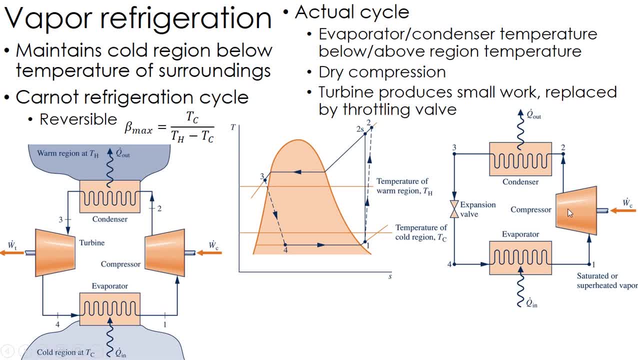 to get heat transfer. the other thing is that compressor needs to be a dry compression which, for the carno that all takes place under the vapor dome. so there would be some quality with the compressor, and a compressor doesn't like to do that. so in a real system we've got to get 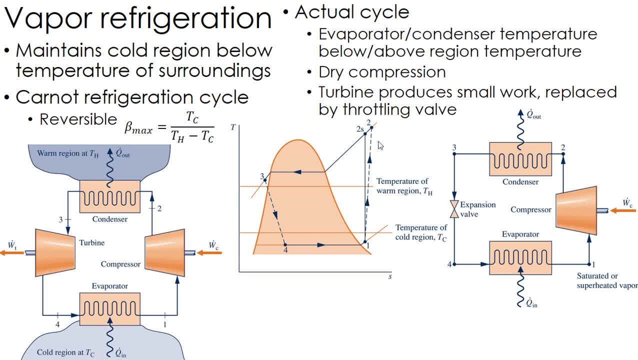 one to two up into the vapor range. so there's that. there there's no liquid because the compressor is not going to compress that liquid very well. i need all vapor at that point. the third one is it replaces the turbine with just an expansion valve. okay, the turbine does not put out much work. 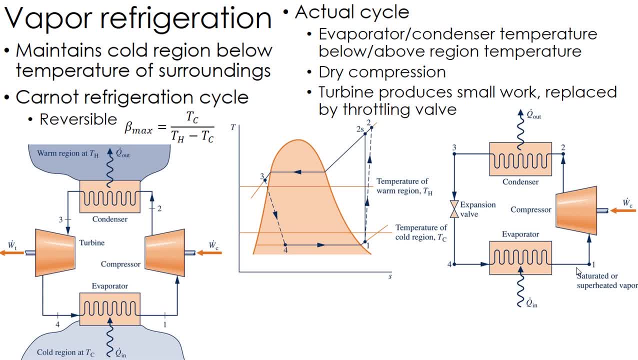 in a carno cycle and the maintenance costs and and upfront costs are so great that it's not worth those costs to get any extra work necessary versus an expansion valve. the nice thing is that makes our analysis much easier and again you can see that the turbo is not going to compress that liquid very well. i need all vapor at that point. 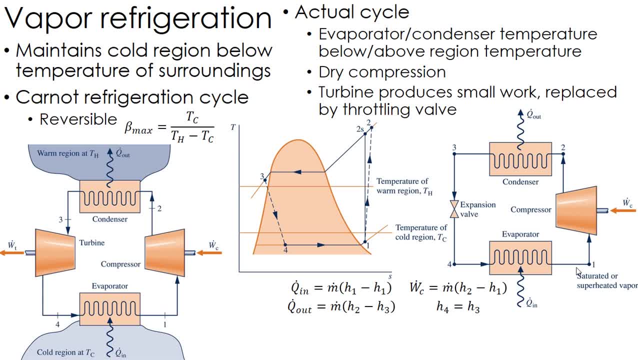 here's our analysis, so i can find q in and q out and work at the compressor, all delta h, but then across that expansion valve there's no work being done, right throttling valve, you know there's no work, there's no heat transfer. so basically enthalpy is constant. so h3 equals h4, okay, so there's really 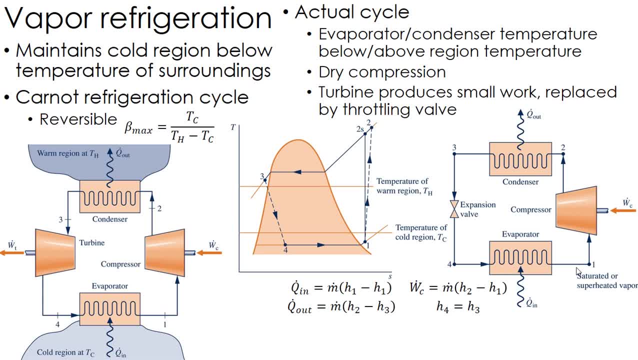 only three states we have to find, because once i find three, i know state four: okay. and then all of the work and qns are just delta h's, which gives us a coefficient performance of qn over the work at the compressor, which is just a relationship of those h's as shown there. okay, so this is the actual. 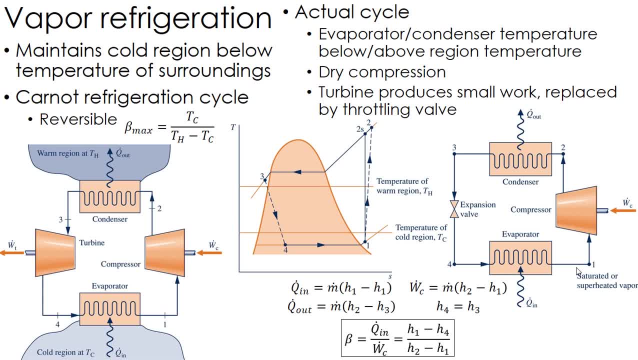 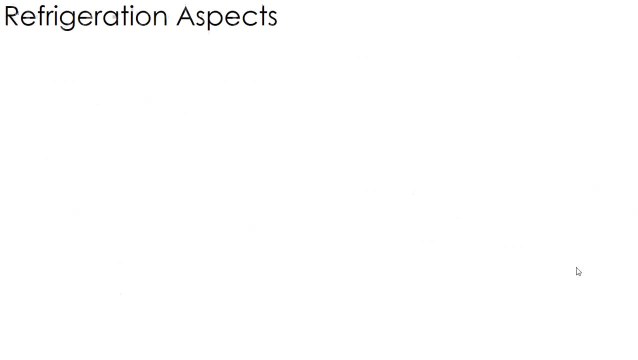 vapor, uh refrigeration cycle that we use. okay, the compressor and expansion valve um dry compression, rather than everything under the vapor dome with the turbine, things of that nature. okay, remember, i do have to have that temperature change in order to get q in and q out. okay, so a few other aspects. 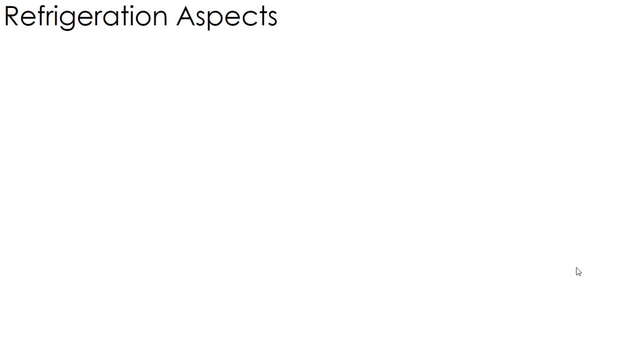 with regards to refrigeration- and i'll refer you to the book if you want a little bit more detail on this. the first is: hey, which refrigerant do i use? you'll notice in the back of the book we've got, i don't know, like four different refrigerants we can choose from. okay, well, the main thing is: 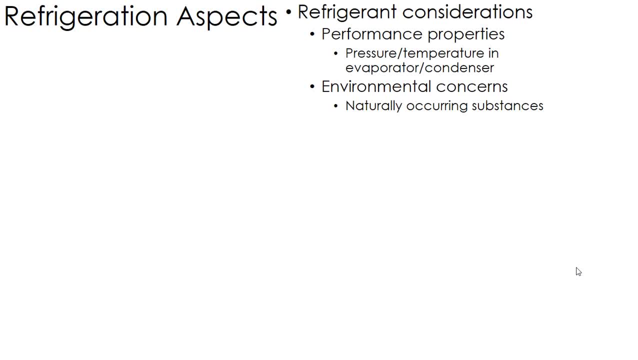 does it perform as we want, which is to say, am i in a temperature range that's useful for the application that i have right? is it a freezer? is it a heat pump? is it a refrigerator? you know? is it just an air conditioner? you know what is it and you need to choose pressure and temperature. 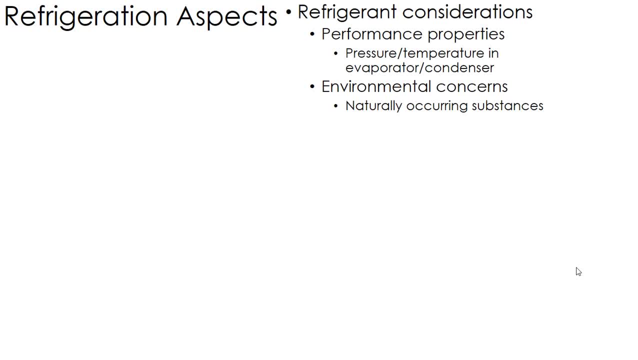 of the evaporator and condenser in order to get that heat transfer that you're looking for. so that's the main consideration when choosing a refrigerant is making sure it's within the ranges that you're interested. we also have environmental concerns. um, you know certain things. 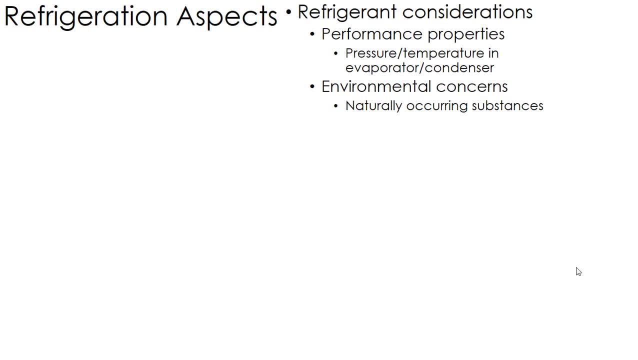 contribute to global warming. uh, certain things are not very good for the environment. uh, in a lot of ways, we're trying to find naturally occurring substances that would be like the propane and the ammonia that we have. uh, for refrigerants, we're moving more to those because of uh, environmental 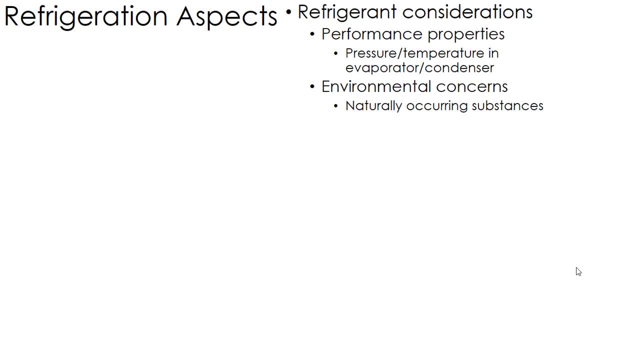 concerns and things of that nature. so those are some considerations that you take in when you choose what refrigerant you're going to use, whether it's our 134a or propane or what have you. a couple other things. first, one is a multi-stage compressing right. so this is basically two. 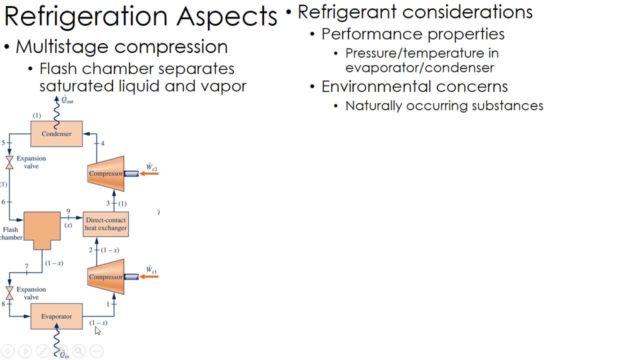 compressors. okay, so, with basically like an intercooler in between going from two to three, you have this, uh, heat exchanger that goes on, uh, basically to decrease the total amount of compressor, that compression that you need now. a key feature of that is this flash. 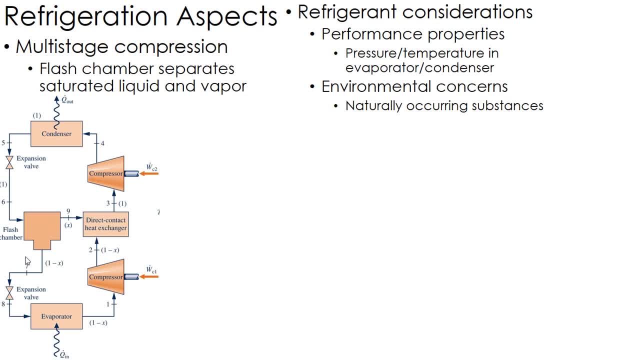 chamber that you see in here, and what the flash chamber does is state six comes in and it's at some quality, and then basically it just separates out the vapor from the liquid, the saturated vapor, saturated liquid, and so saturated vapor goes out at nine. saturated liquid goes down at seven. 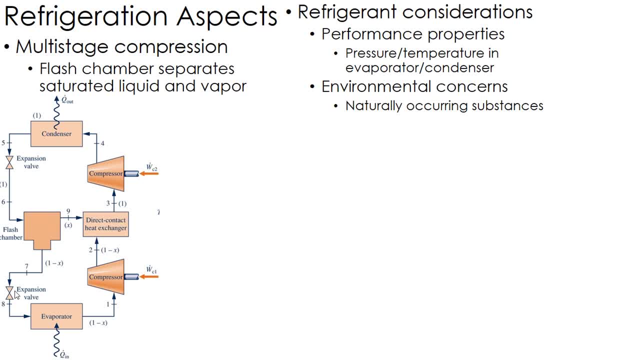 and the amount just depends on what. the quality is right. so if the quality is ninety percent, ninety percent of the mass will go out as um vapor, ten percent will go out as saturated liquid. okay, but again, this is the sort of setup where i've got kind of multi, two compressors that i'm 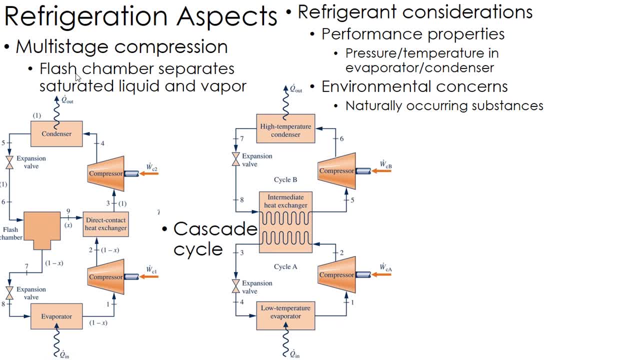 doing here? um, another one is cascade cycle. this is basically two refrigerators on top of one another, and we've done this several times now with the power cycles, where basically q out of one is q into the other. okay, so again we've got two compressors here. generally i'm going to have 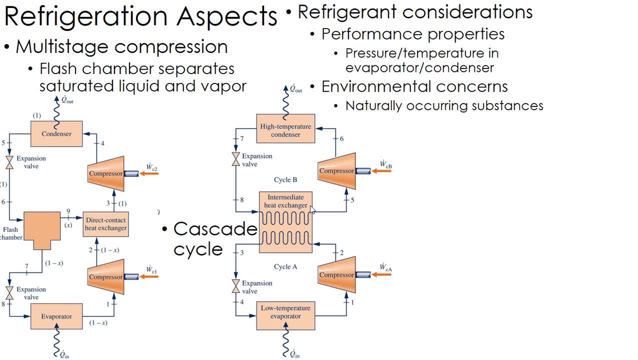 probably different refrigerants. but again it's that whole idea of, hey, why dump it out? why don't i dump it out and get a little bit more performance, kind of idea here we did a lot of that with both vapor and gas power cycles- the other one that we want to talk about just a little bit, and again i'll refer your book if 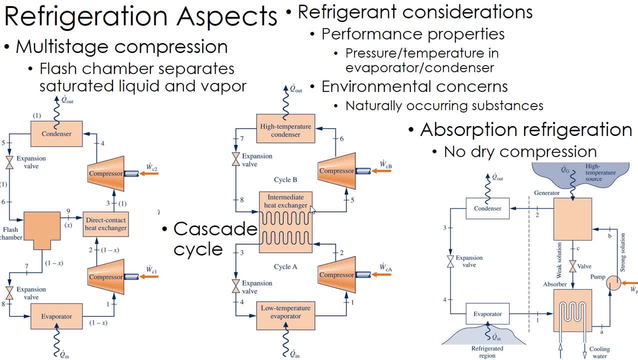 you want to read a little bit more about this, but that's absorption, refrigeration and basically, rather than use a compressor, it uses this whole kind of pink thing over here. okay, where, instead of the compressor, which requires a lot of work, we're going to use a pump, which requires a lot. 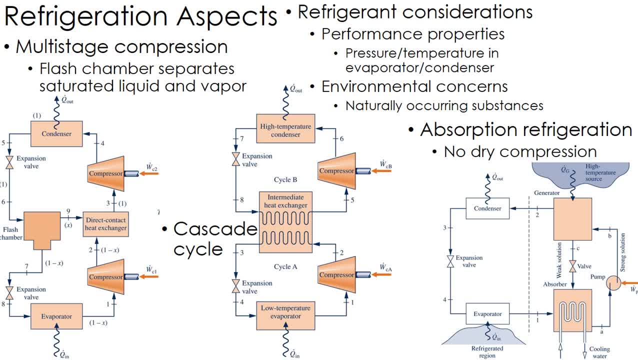 less work. okay for the pump to work out, though it all needs to be a little bit more to be a liquid. so then, rather than- you know that- dry compression, i actually want to go all the way down to liquid, and that's why i have this cooling water coming in here. 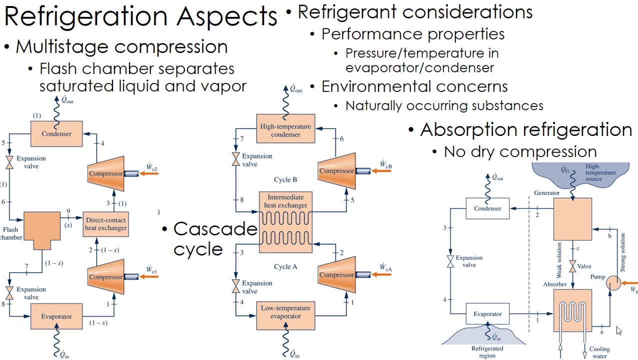 reducing it down from some sort of quality all the way down to probably saturated liquid, so then i can put it through the pump and then continue on through. so again, rather than that compression, we use a pump, which requires less work, but then i do have to add a little bit extra heat.